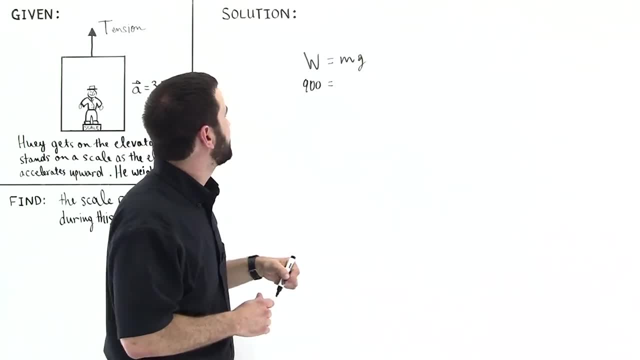 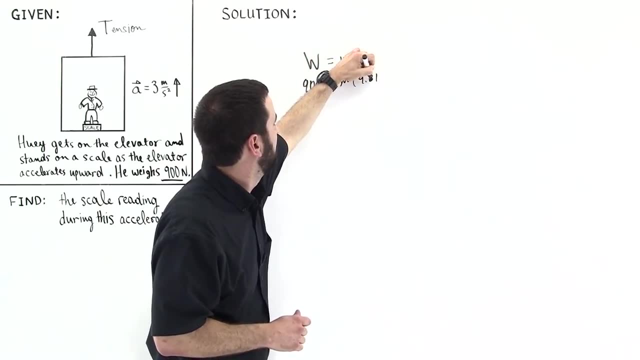 incidentally, It's a little bit more than 200 pounds, And so mass times acceleration due to gravity is 9.81.. And then the mass will be equal to 91.7 kilograms. Dividing by 9.81 on both sides, we get 91.7 kilograms. 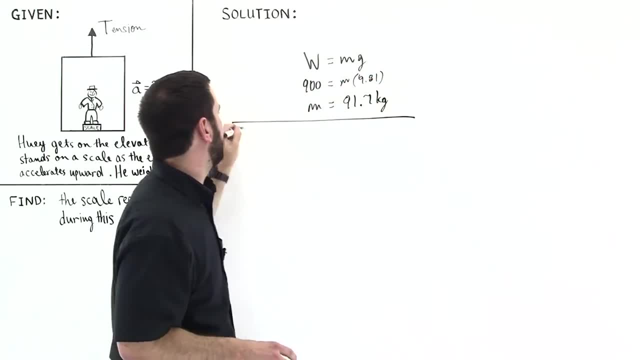 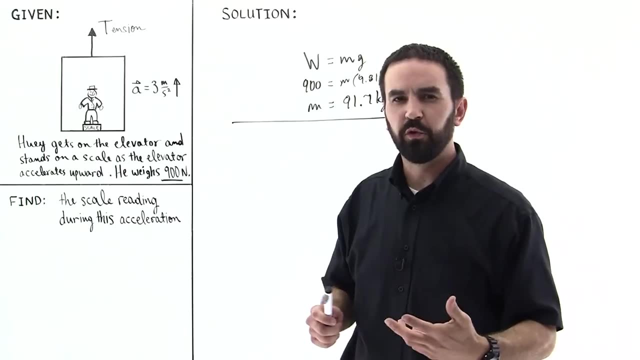 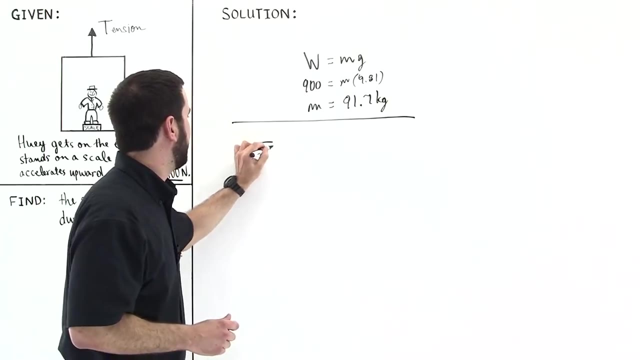 Like so Okay, so let's take a look at this situation And we're going to draw a free body diagram, And we're just going to draw the free body diagram of Huey himself, right, without all the external distractions. And that's what a free body diagram is. It's a 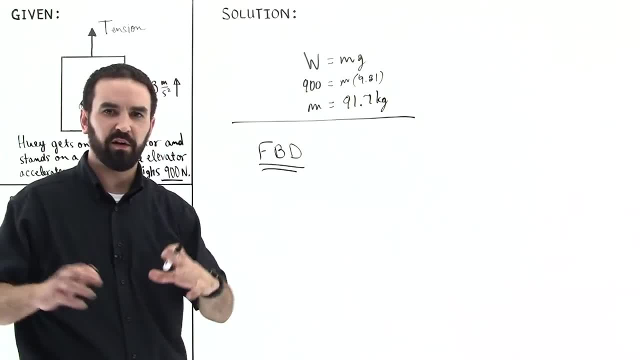 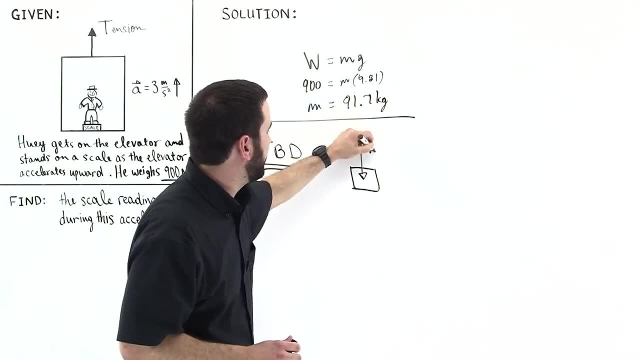 picture of the object being analyzed without all the external distractions. So we're just going to draw him as a box And we have Huey's weight weighing him down like this, And then there is a force, a normal force- we'll call it pushing up- And this normal force is from: 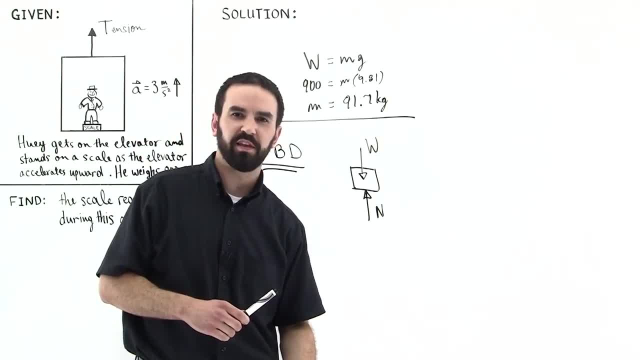 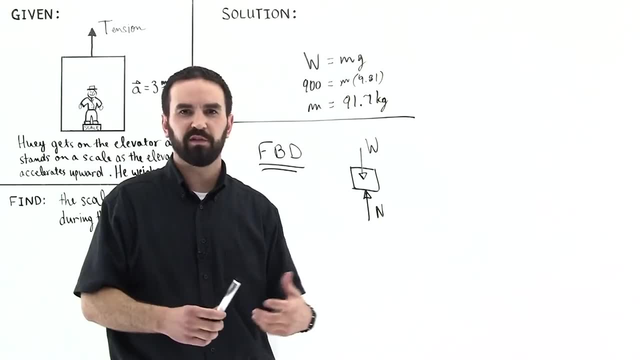 the scale right. The scale is pushing up underneath his feet, And so whatever this normal force reads, that is what the scale reading is. The scale reading is the normal force. So then he's accelerating upward. We also have to include the acceleration on the. 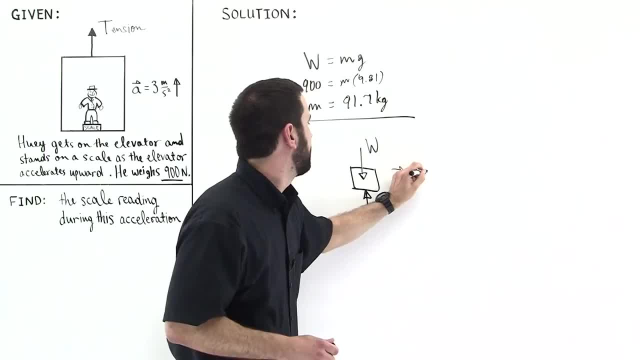 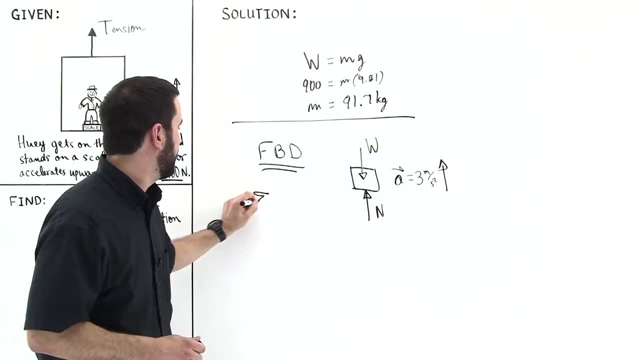 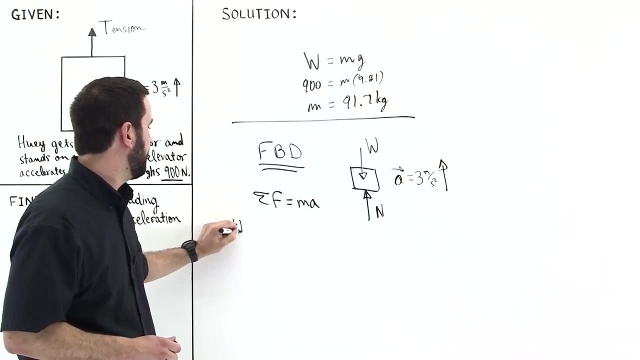 free body diagram. So he's accelerating upward at 3 meters per second squared. I'm going to write upward like: so right, So we'll apply Newton's second law. We say sigma F is equal to mass times acceleration. We have the normal force pushing up, So plus N, the weight opposing. 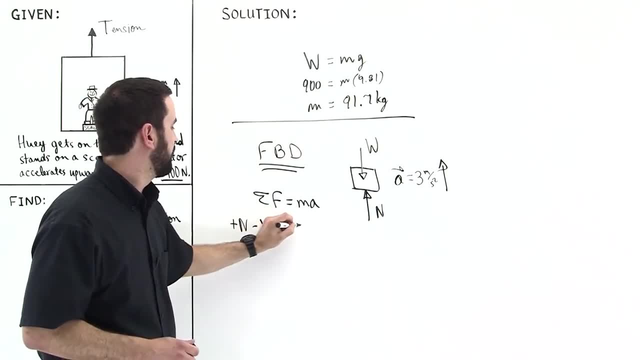 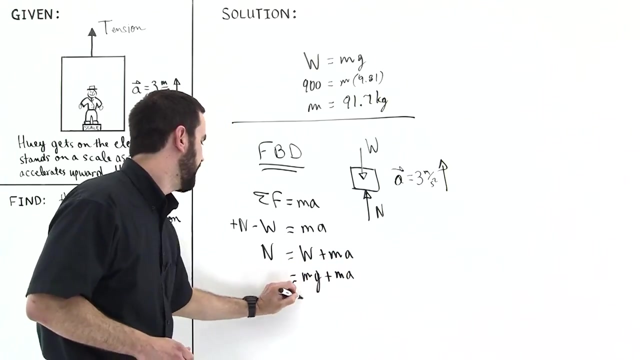 it minus W equals mass times acceleration. So bringing the weight over, adding the weight on both sides, we get the normal force is equal to the weight plus the mass times acceleration. So weight is equal to mg. right, So we can express that as mg And then factor an m out. 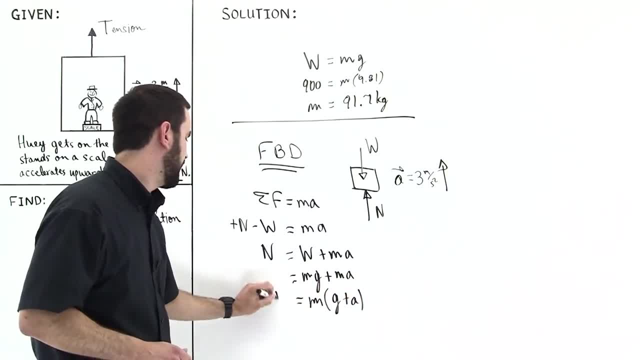 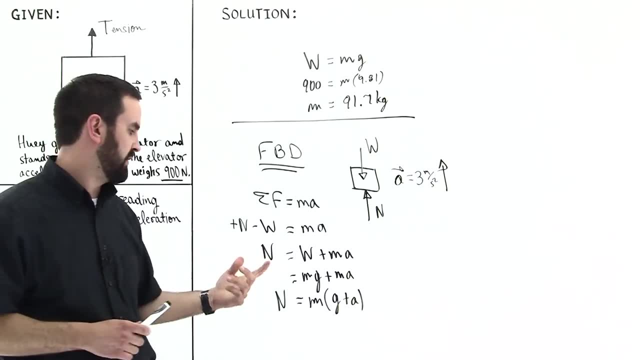 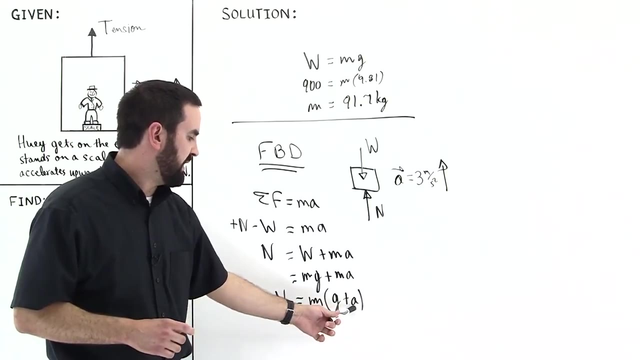 to see more clearly what's going on And we get the following: The normal force is equal to the mass times, the sum of the acceleration and the gravity right, The gravitational acceleration. So if this is big right, then the normal force is big right And you can think about it in the following: